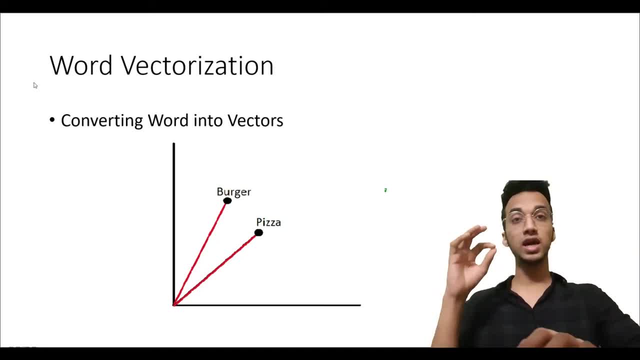 what is the significance of words having a direction? So that is very important to understand. For example, you can see there are two words, burger and pizza, And when you represent them as vectors, they'll have a direction right And because of the sense of direction, you can. 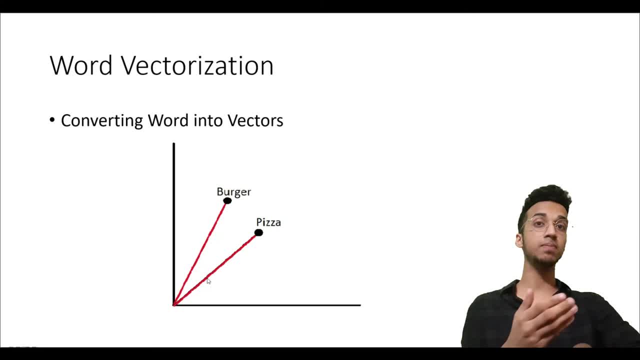 establish how similar these two points are. for example, burger and pizza should be close to each other since they're food items, right? So that is where concept of direction also comes in. But just to understand how we're going to do things, you can think of it as converting words. 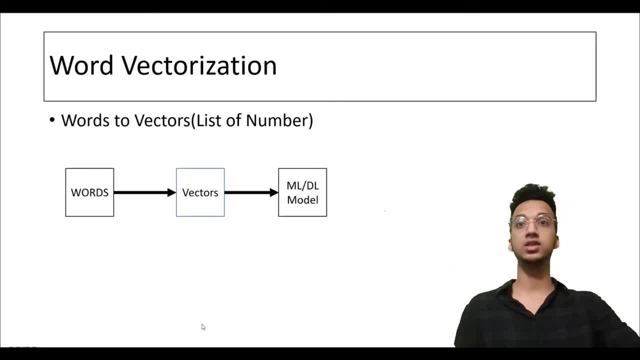 into a list of numbers. Right For all practical sense. So words will be converted into vectors, or it will be converted into a list of numbers, And these numbers are going to be given to the machine learning model. Now question is: how do we convert them into numbers, And there are few popular methods of. 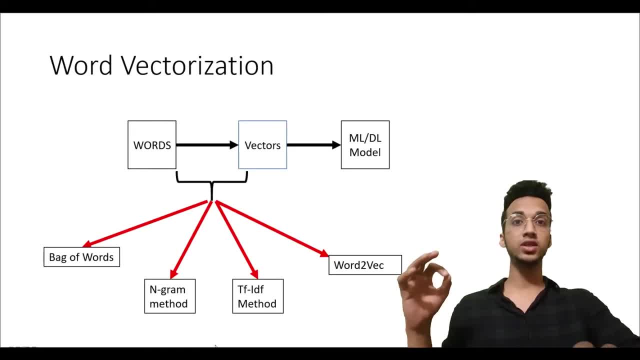 doing this, which we're going to discuss in different videos. So these are the four popular methods of converting words into numbers. In this video we're going to address bag of words Right. So if you go to any data science interview or natural language processing based, 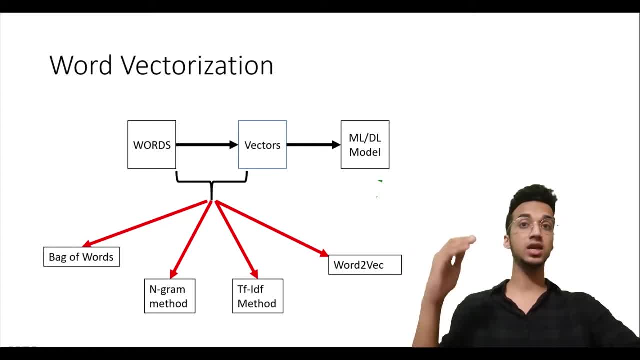 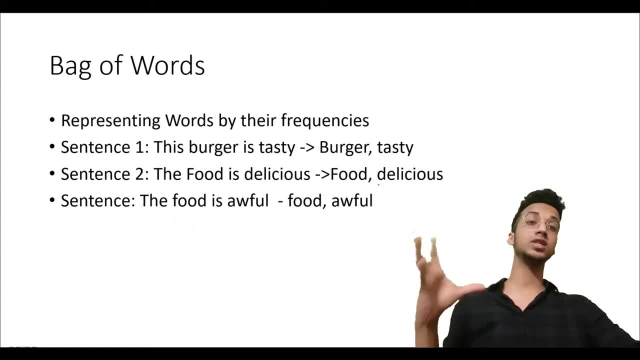 interview. it is important you know these four methods at least, and the drawbacks of each one as well, And what are the advantages of different methods. So let's look at bag of words. It's a very simple concept And it represents words by their frequencies. Right, It's a way of 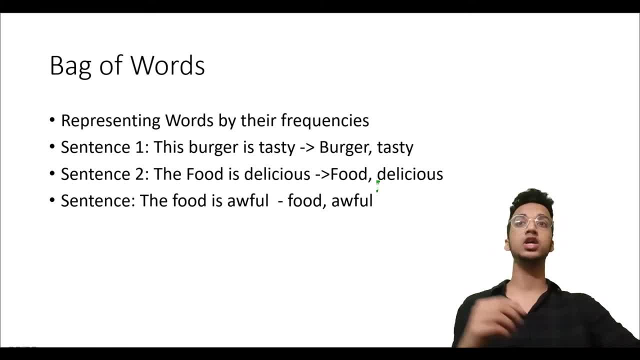 representing words by the frequency by which they're occurring. So let us look at these three sentences. right, The burger is tasty, the food is delicious, the food is awful. And you have to convert these three sentences into numbers which you can give to a model. So first, 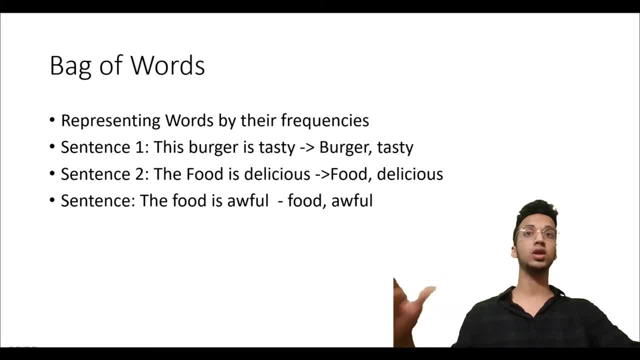 of all, in most processes you're going to remove stop words right As we talked about. words like this is are not really significant, So the final words that you would probably supply to the model could look like this: burger comma, tasty food comma, delicious food- come off. 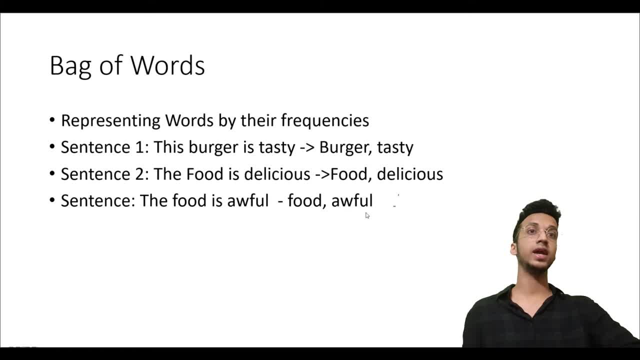 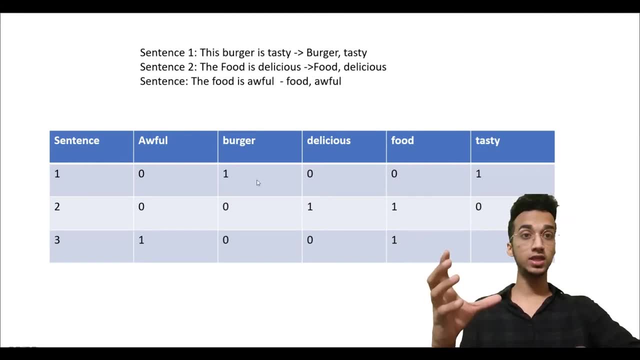 And these are the words which are determining the meaning, Right? So let's look at how we could represent this, Right? So, basically, we represent each word by the frequency in which they're occurring, And you can represent them in a matrix like this. So, basically, you're. 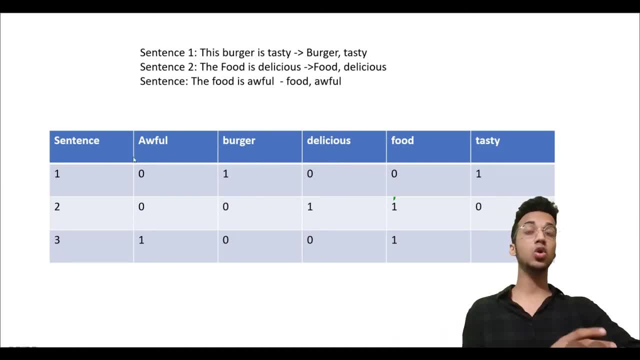 going to have different columns, which are also called as features. different column for each word occurring in the document And for representing a particular sentence will simply change the corresponding frequency of the word. For example, sentence one was burger tasty right, So the 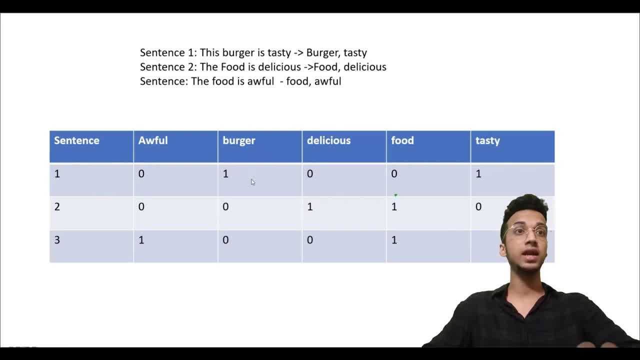 corresponding column to burger is represented as one and tasty as one rest. all are zero. Similarly, food is delicious, for sentence two would become delicious, and food are represented by one, rest or zero. Similarly, food awful is represented like this: Right. And this is called as binary bag of words, because everything is in zeros and ones. 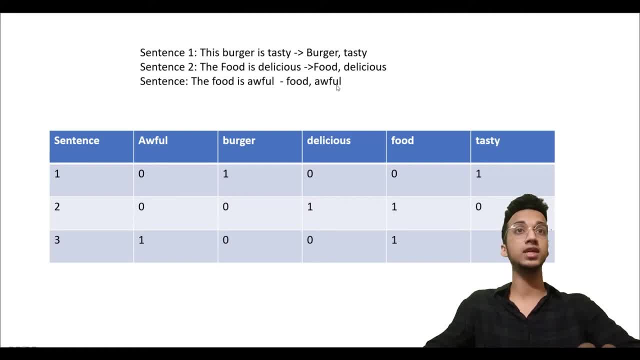 For example, if a particular word was occurring twice- say burger, tasty, burger- then the particular column for this burger will become two, right, And it would be a normal bag of words, Right? So it's very easy for each word representing the frequency by which occurring. 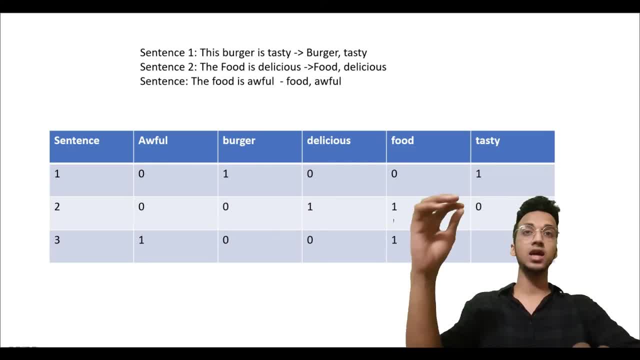 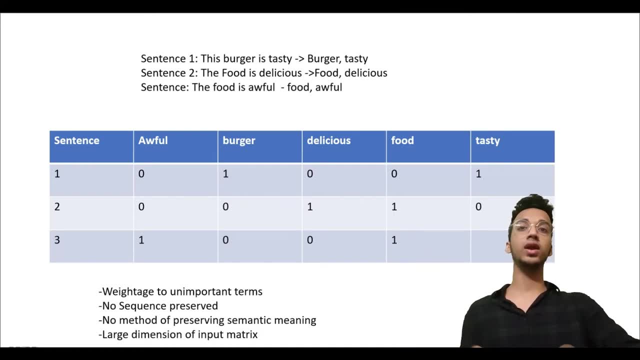 And this is the list that you're going to supply to the model- And there are a few drawbacks of this which you should be able to spot right off the bat, For example. now, the first disadvantage is that weightage is given to unimportant terms, For example, 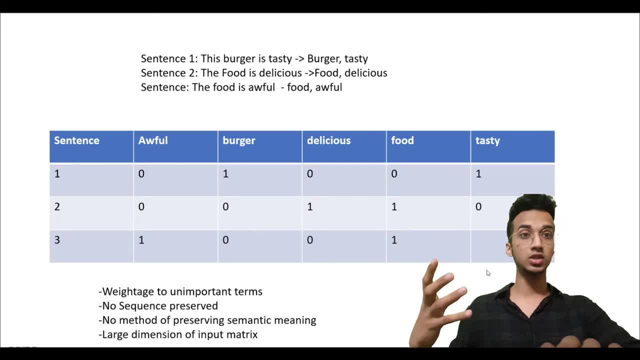 burger is tasty, right? Let's say you want to do sentiment analysis. what is the customer saying about your burger? In this case, tasty is very important, right? Burger is not as important what the customer feels is important. So in this case, burger and tasty have the same importance. 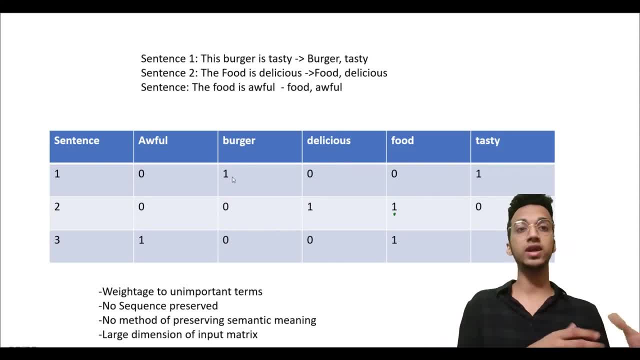 they have same weightage. So what is more important does not get more weightage And some commonly occurring words like this: and, or. if it's not removed, they'll occur a lot. they'll get a very high frequency and the model will get fooled into. 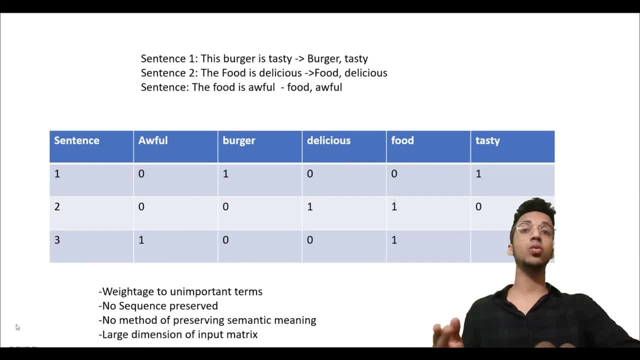 thinking that those words are important, And another disadvantage is that no sequence is preserved. Mostly these features are in alphabetical order- at least in Python implementation it is, but there is no order of the original sentence. For example, the sentence are you smart and sentence you are smart will have the same vector representation because they 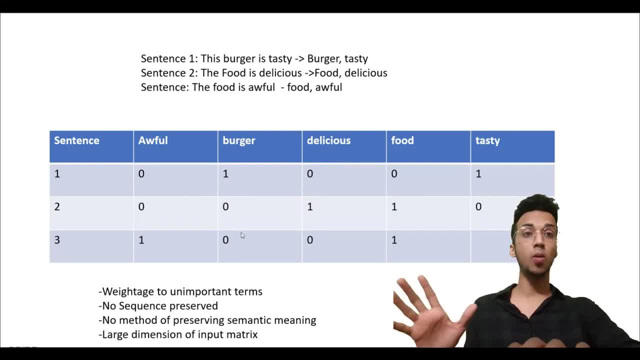 have the same words, But these two sentences are completely opposite of each other, Right? So sequence is not preserved in bag of words. Again, there is no method of preserving semantic meaning, So basically, there's no sense of the meaning as well. For example: 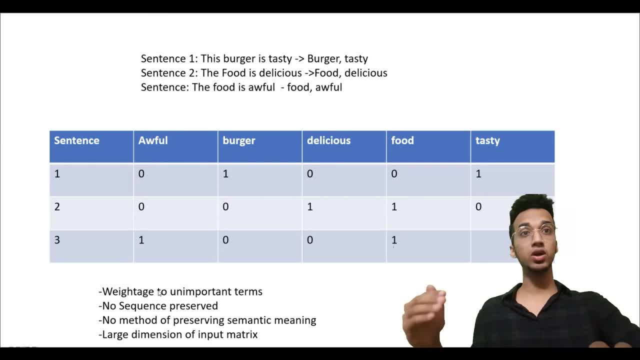 these two sentences: food is delicious and burger is tasty. There are very similar sentences, right, They're very closing meaning. they're both conveying the same sentiment. So machine learning models to understand that, But with this bag of words approach it has no way to do that. 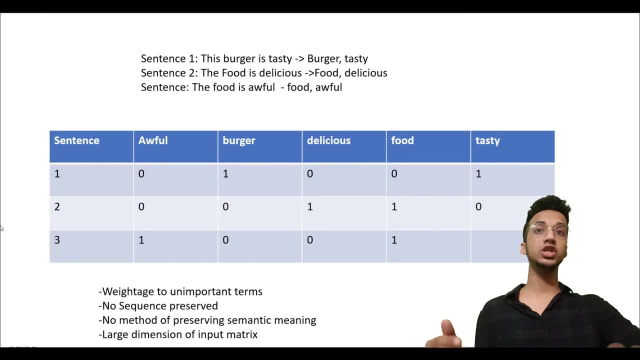 Right. For example, if you see food is delicious, which is a sentence, and food is awful, These two sentences are completely opposite of each other, But the machine learning model does not know that. Instead, it will think that these two sentences are similar. 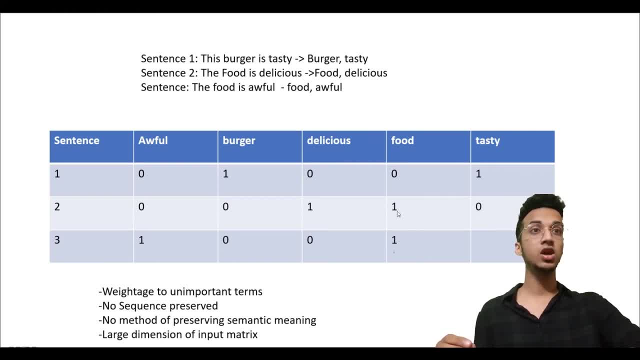 because they have the same number, they have the same frequency for the feature food Right, So semantic meaning is not preserved. Also, you can see that this dimension can become very, very large. So the number of columns in this matrix will depend upon the total number of words in the 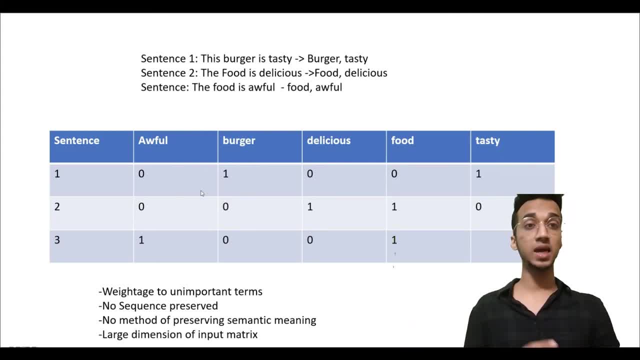 document. As a result, in large documents this number of words will be larger than the number of words in this matrix can be very, very huge, which we want to avoid generally, Right. So these are the few major disadvantages of bag of words And because of these we use different. 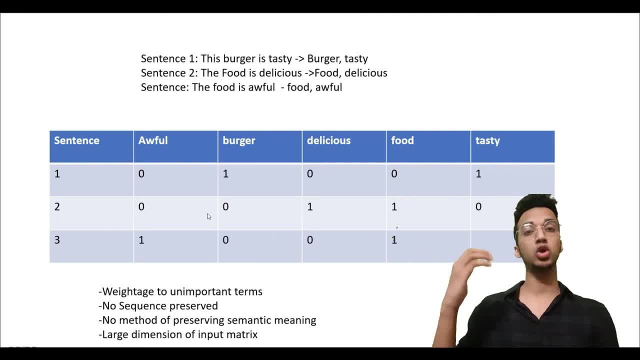 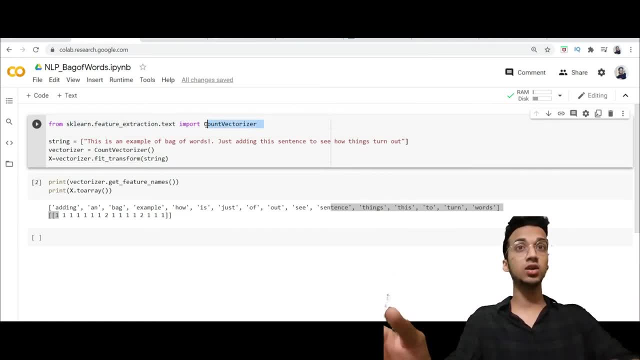 approaches now, But still, for the sake of completion of this topic, I'm going to show you how to implement this in Python now. So this is going to be very short coding video. So in this code we are going to use sklearn to import a function called count vectorizer. 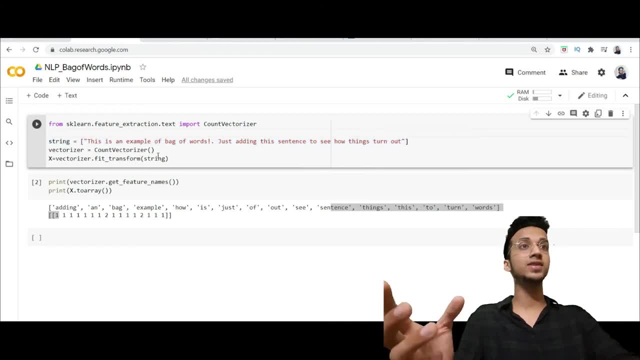 which is a very handy tool for doing bag of words. So let me just give you an example. See, this is an object, right, and I give it the name of vectorizer, And you basically use the function vectorizer, dot, fit, underscore, transform, and it will automatically create, first of all, a list of 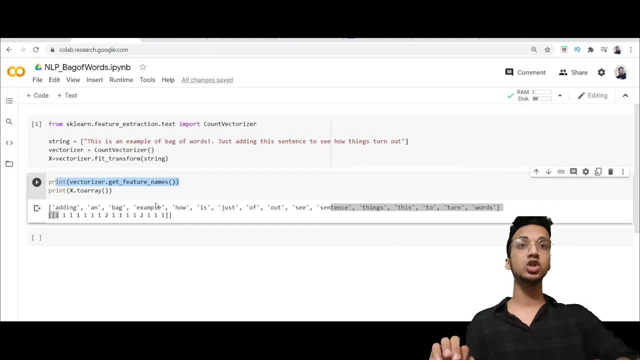 all the features and the particular frequency Right. So here I'm printing all the feature names and to print the actual list of numbers I call the function to array And you can see the result. these are all the features in the particular sentence right, with the corresponding frequency.